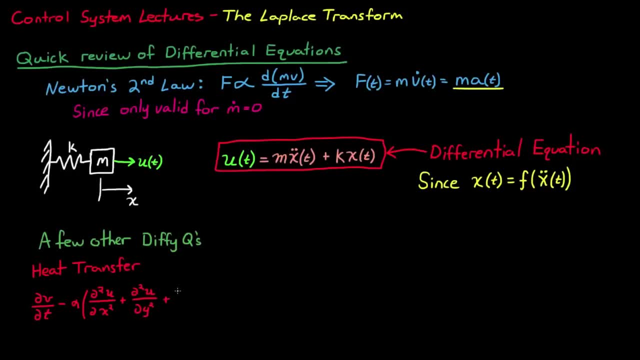 There's the heat transfer equation, and this describes the distribution of heat in a room, And this describes the distribution of heat in a region over a given time. Another is the radioactive decay equation. that states that the rate of decay is proportional to the amount of material. 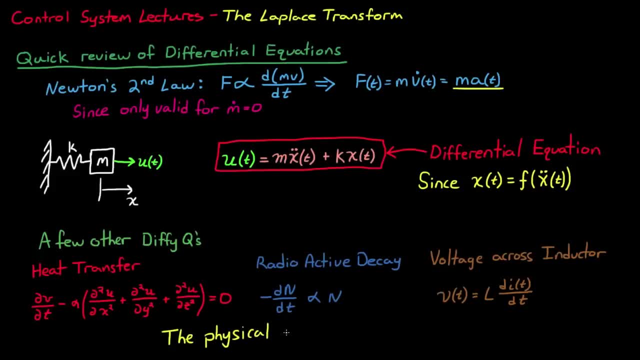 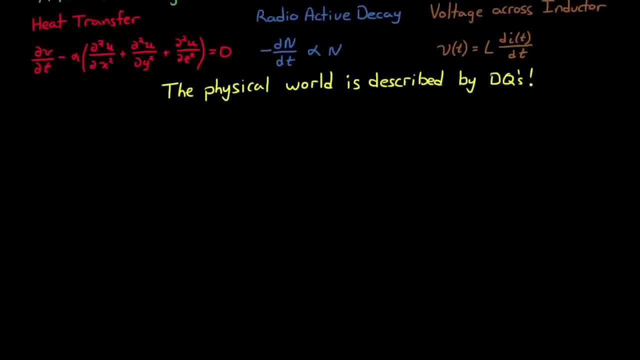 and the voltage across an inductor is proportional to the rate of change of current. So you can imagine why differential equations are so important. It's because the physical world is described by them, And if you've taken differential equations as a class, then you know that their solution can only consist of exponentials. 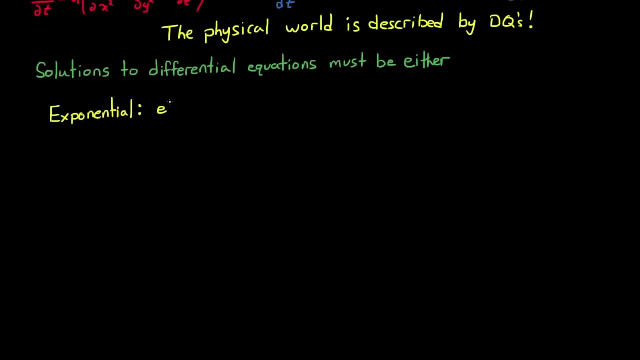 which are e raised to a real number, and sinusoids, which is e raised to an imaginary number, Although, just to make a point here, I'll refer to the sinusoid as just sine of a, t. Now, the reason this is true is because the derivative of an exponential is just a scaled version of itself. 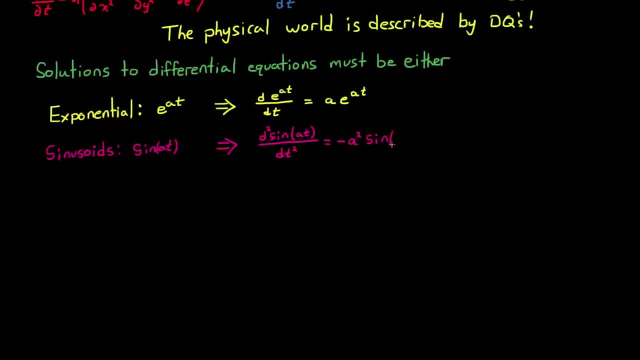 and the second derivative of a sinusoid is the negative scaled version of itself, And you'll notice that the original function still exists in the solution and these two types of functions are the only functions that exhibit this behavior. So when your equation is a function of a signal and some order of its derivative, 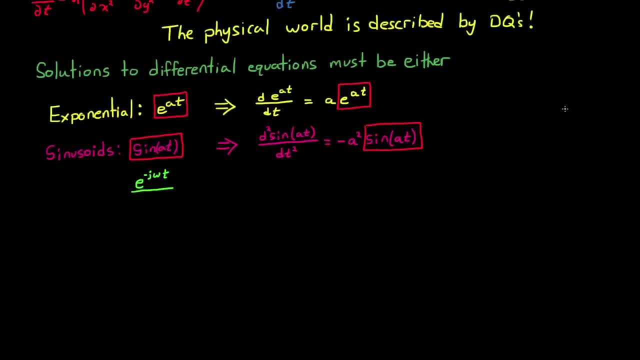 you automatically know that the solution must contain either a sinusoid e to the negative j, omega t or e to the a t, where a is a real number, or a combination of these two functions. Alright, now let me start trying to tie this all together. 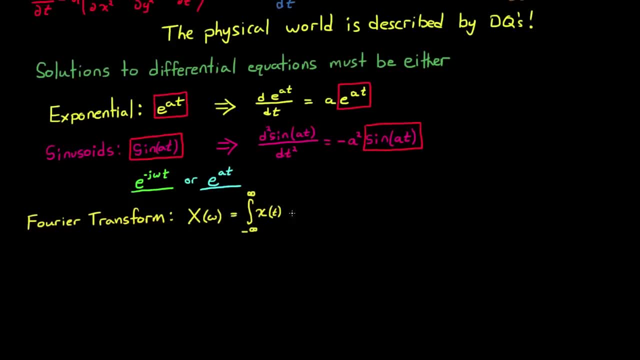 We'll start by looking at the Fourier transform. Now, when you see the Fourier transform, you should notice that it analyzes signals in terms of sinusoids. This is called the frequency response and is a general approach to move from the time domain to the frequency domain. 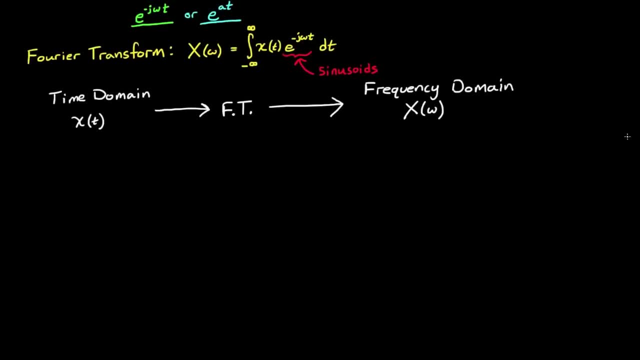 The problem, though, is that this is a little too restrictive when dealing with differential equations. I mean, where's the exponential term? In my videos on the Fourier transform, I explain that the way to move from the time domain to the frequency domain is to take a time domain signal. 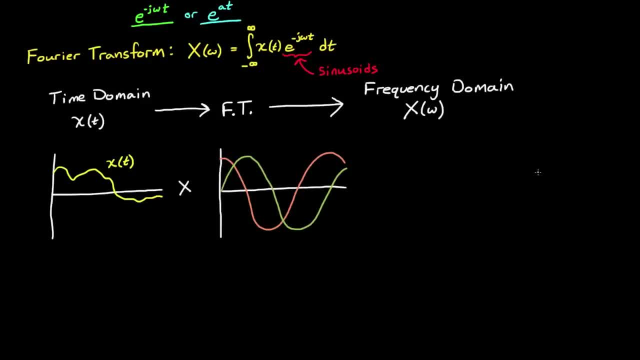 pre-multiply it by a sinusoid e to the negative i, omega t, which contains both imaginary and real sinusoids, and then sum the remainder across all time to get the frequency domain information. But what if we wanted to start thinking in terms of exponentials and sinusoids? 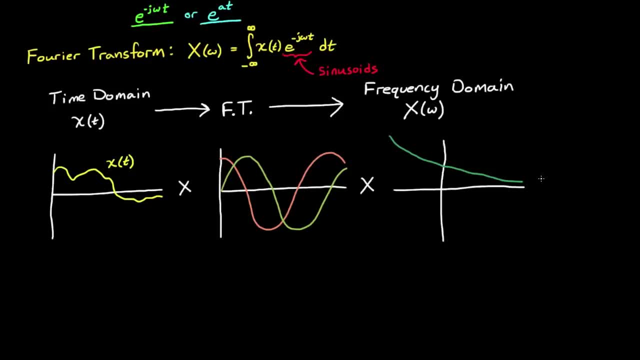 Then couldn't we also pre-multiply it by an exponential term as well? Here we're going to start with the time function x of t. We'll pre-multiply it by an exponential term, e to the negative sigma. Then we'll treat that function as our new x of t. 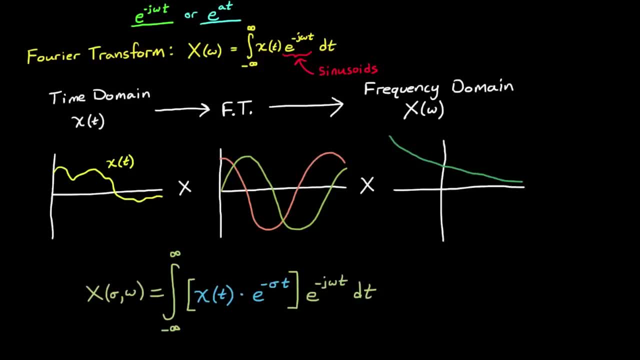 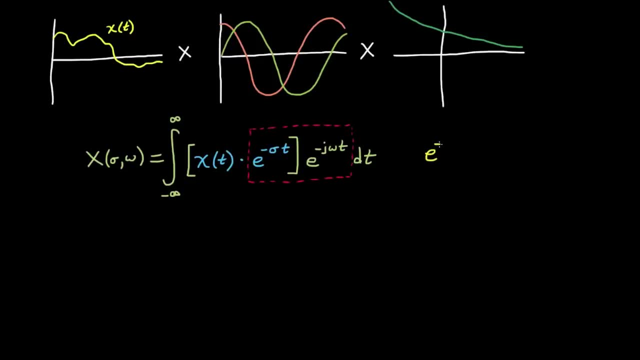 Now we can take the Fourier transform of this to see what it gets us. Now, at this point, we can combine these two different exponential terms into a single term, and this term is e to the negative sigma minus j, omega, all of it times, time. 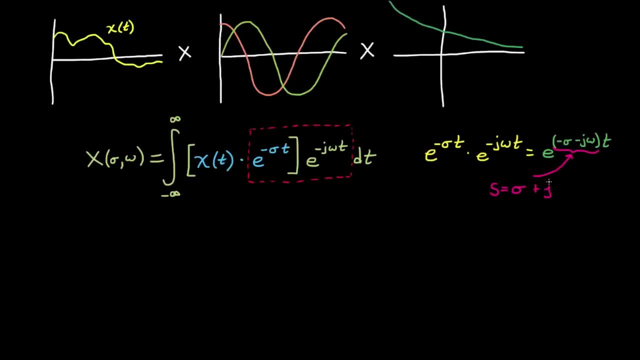 At this point we designate the variable s as sigma plus j, omega, And s is a complex variable because it contains a real portion, which corresponds to exponential responses, and an imaginary term, which corresponds to sinusoidal responses. And substituting this variable s into our equation, 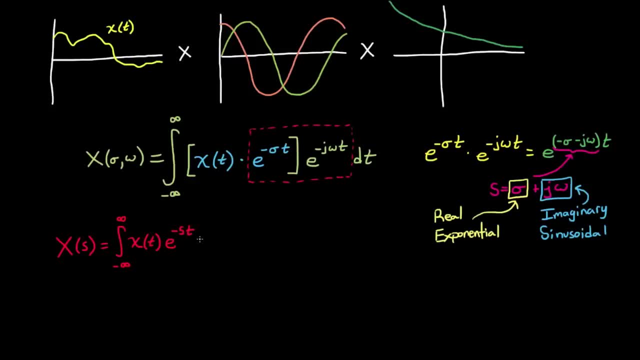 gives us the standard form of the Laplace transform, And it's this transform that moves us from the time domain to the s domain and back. So let's see if we can get a better idea of what the Laplace transform is doing by looking at it graphically. 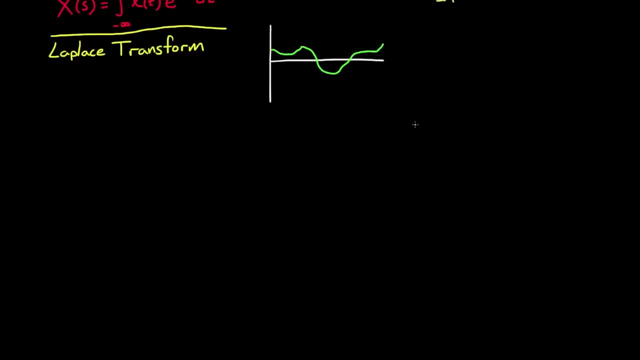 We'll start with any arbitrary time domain function f of t, Then we'll pre-multiply it by an exponential term. in this case, let's say sigma equals 0, and then take the Fourier transform of the result, Since sigma was 0 and e to the 0 is 1,. 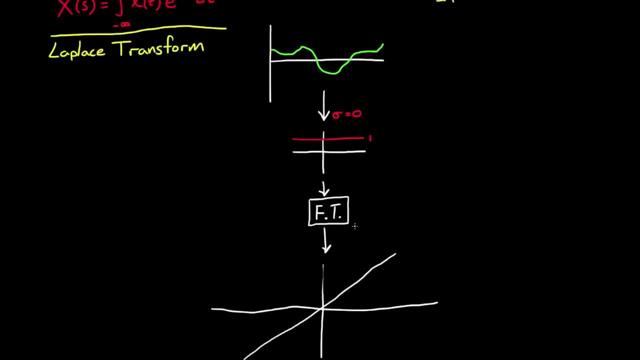 this is identical to just taking the Fourier transform of f of t And we can plot the result of this along the sigma equals 0 line in the s plane, But so far we only have a single value of sigma and we need to populate this entire plane. 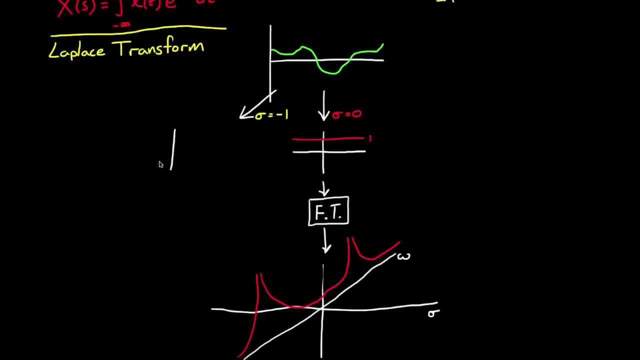 So now let's take a second value of sigma, let's say at negative 1, pre-multiply it by that exponential, then take the Fourier, transform and now place that result along the sigma equals negative 1 line in the s plane. 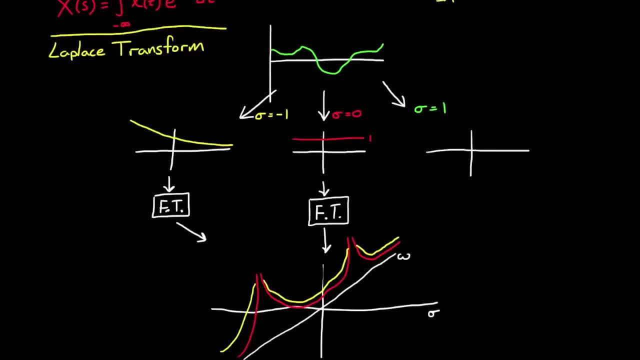 Now we can do this a third time at sigma equals positive 1, pre-multiply it by that exponential, then take the Fourier transform and then write the results of that at the sigma equals 1 line in the s plane. Now of course it would really be impossible to do it this way in real life. 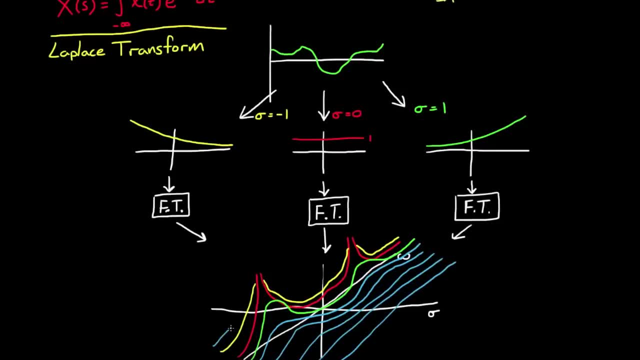 but that's the nice thing about the Laplace transform is that we don't have to perform these steps one at a time. The standard equation that I wrote earlier for you fills in the entire s plane in a single step, But remember that s is a complex variable. 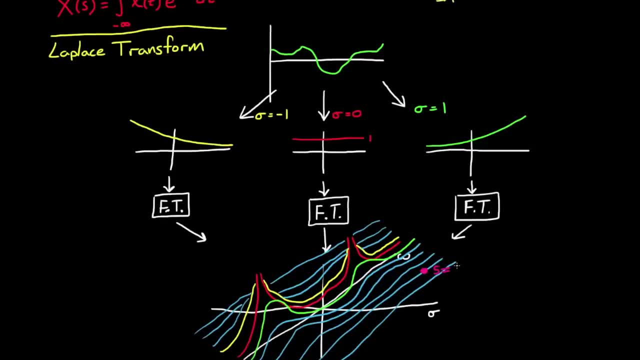 that describes a location here in the s plane. It has a real value- sigma- and an imaginary value- j, omega. But the location isn't the only thing that's complex. The value at that location is also a complex number. It has a real component and an imaginary component. 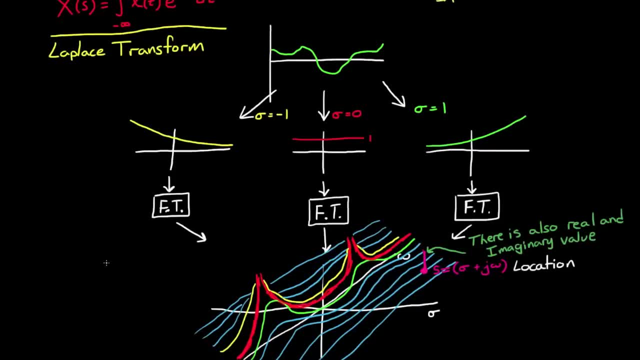 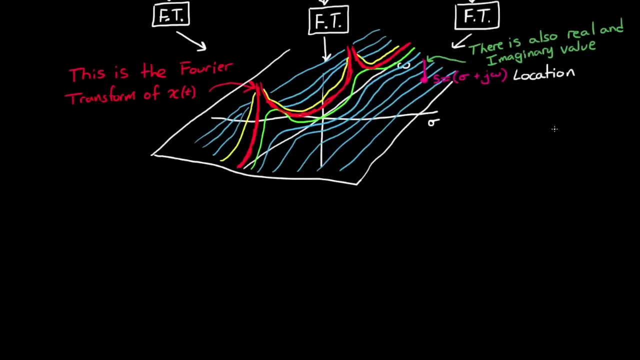 And this value relates back to the phase and amplitude, just like the Fourier transform. Another thing that's interesting is that if you look at the sigma equals 0 line in the s plane. this is exactly the Fourier transform of the function. Now, I drew the s plane here askew on purpose. 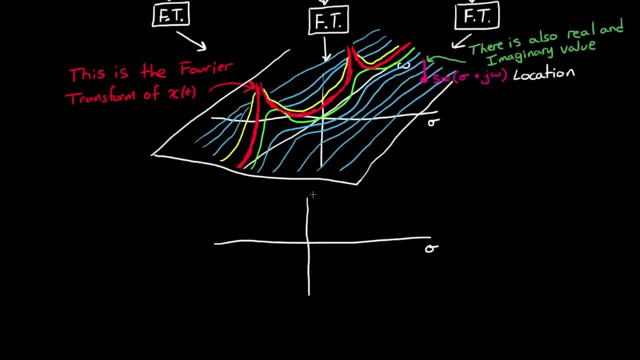 so that you can see the contours of it. However, normally when you see it, it's just two-dimensional, with sigma on the horizontal axis and omega on the vertical axis, And we normally don't care about most of the graph. We really are only concerned with where the peaks or the poles are. 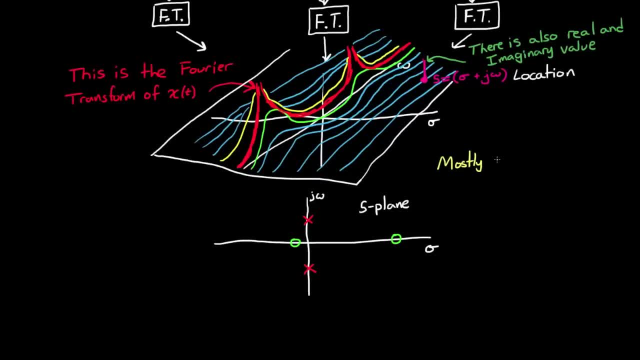 and the valleys or the zeros Poles are marked with an x and zeros are marked with an o. Now I've drawn the x's in the correct spot according to my contour plot above, but I'll just add some zeros in here. anywhere 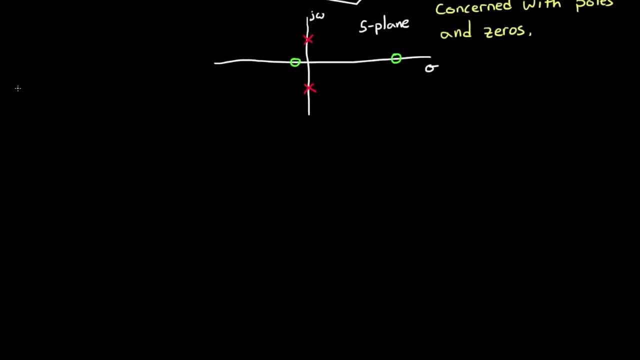 just to show you what they look like, But don't let that confuse you. So the question now becomes: how does this help us understand the linear system that's governed by differential equations? Once again, let's answer this question graphically. Let's take a linear system that consists of an RLC circuit in series. 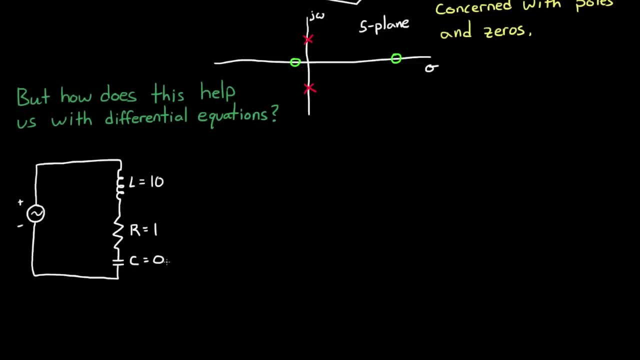 It can be shown that the differential equation for this system, from voltage input to current output, looks like this large differential equation. And if I choose R equals 1,, L equals 10, and C equals 0.1,, then the impulse response looks like this: 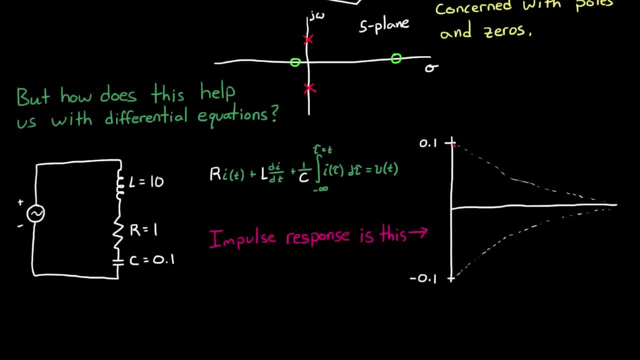 an exponentially decaying sinusoid. Now, to get this impulse response, we could have just solved the differential equations directly, or you could have measured the impulse response of some physical apparatus directly with some test. But now that we have the impulse response here, 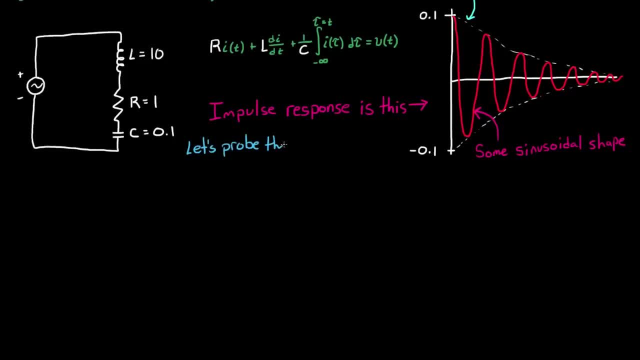 we can probe it using a bunch of different exponentials and sinusoids using the Laplace transform to see what we get out. Each set of exponential or sinusoid- real and imaginary values corresponds to a specific location in the s-plane. Basically, what we're doing is multiplying it by e to the negative st. 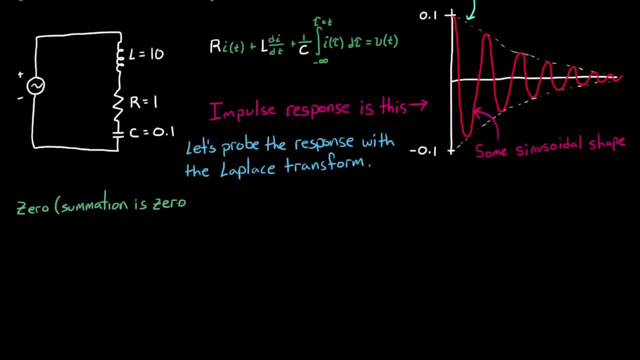 and then integrating the result and seeing what that result is. Now we're looking for two specific outcomes: One where the summation of the area under the curve is 0, it cancels out as you go to infinity. And then the second outcome is when the summation 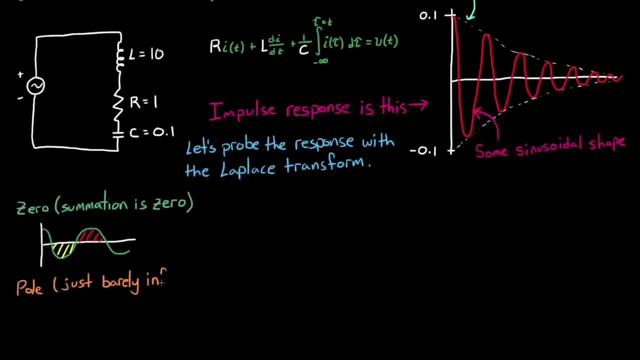 is ever so slightly below infinity. The first is called a 0, and the second is called a pole. Now, summing to 0 is something that's easy to understand, But what does just barely infinite mean? Well, take this orange signal with constant amplitude. 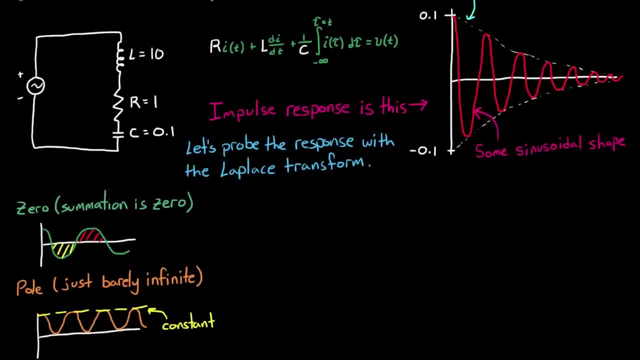 but instead make the amplitude get ever so slightly larger, Then the limit of the area as time approaches infinity is unbounded and infinite. However, if the amplitude is ever so slightly decreasing, then the limit of the area as time approaches infinity is finite, although unfathomably large. 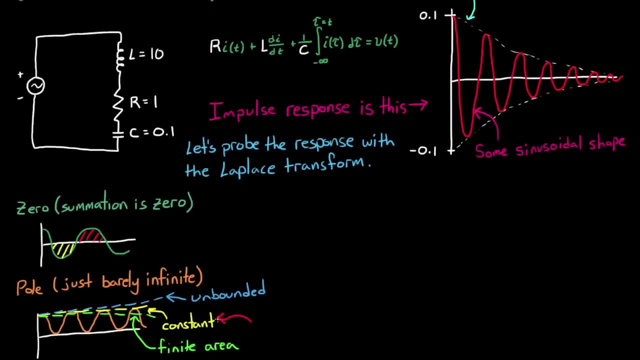 Just between these two values is something I'll call barely infinite, between just a really, really large number and an unbounded infinite number. Now any value of s that doesn't cause either a 0, a summation to 0, or a pole, a summation of just barely infinite. 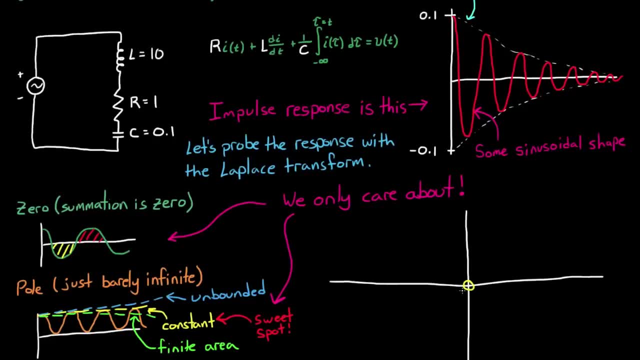 is, in general, just some boring number that we don't really care about, And so we'll just look at poles and zeros. Now, if you'd used the Laplace transform to probe our impulse response at all values of s, then you'd find that we had two complex poles. 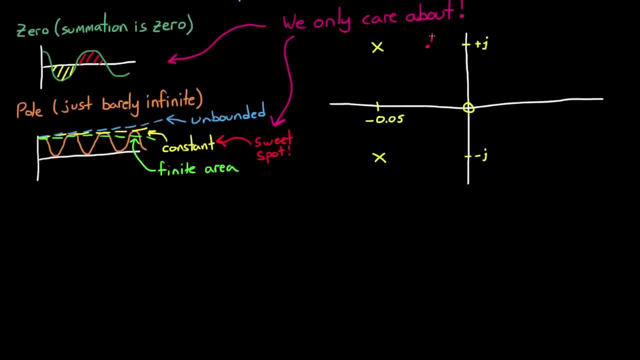 in the left half plane and a 0 at the origin, like I've drawn here. But to illustrate how the Laplace transform works, let me just pick a few spots and we'll go through it one by one. Let's start with a and its complement, a prime. 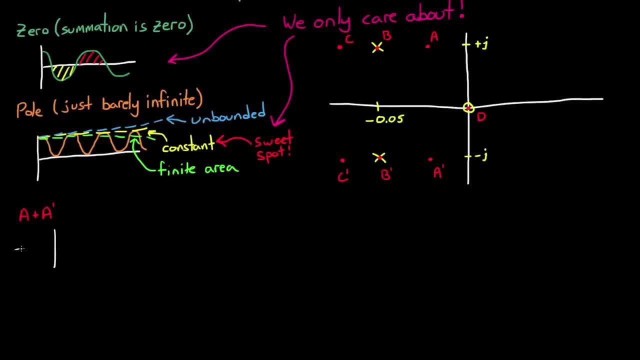 then b and b prime, c and c prime, and then d. Let's start with a and a prime, which decays much slower but at the same frequency as our impulse response. I'll draw the impulse response on top of it in yellow. 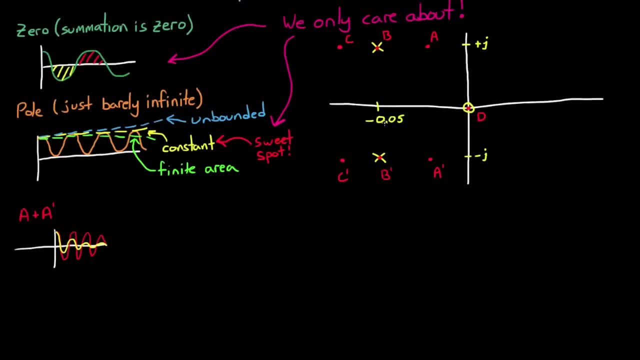 You can see that it's decaying faster. And if you multiply these two equations together and then sum up the result, you're going to get some boring number that's neither a pole nor a 0. But if you move from the a's to the b's, 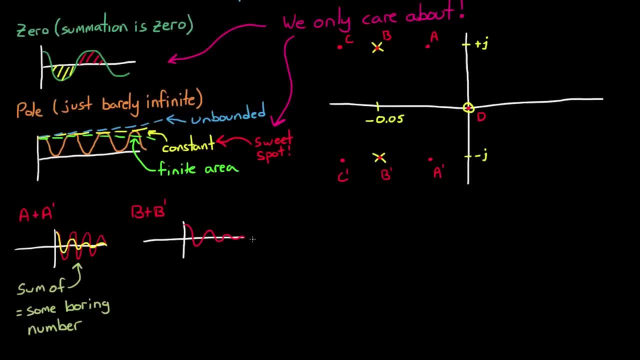 which just makes it a faster decaying probing signal. then our probing signal matches our impulse response exactly And if you multiply these and sum them up you're going to get a very, very large number, just barely infinite. Now, if you pick point c, 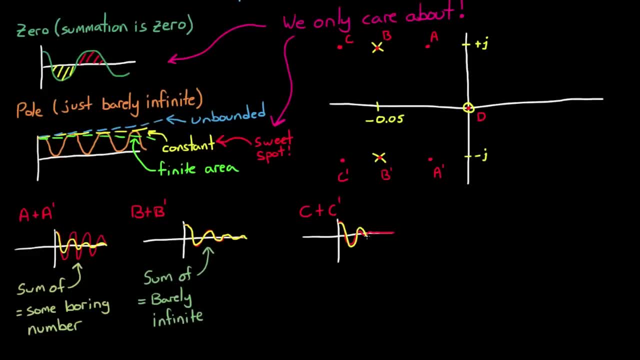 where the probing signal decays faster than our impulse response, and you multiply these two signals together and sum them up once again, you're just going to get some boring number that we don't care about. And then, finally, if you go to d, 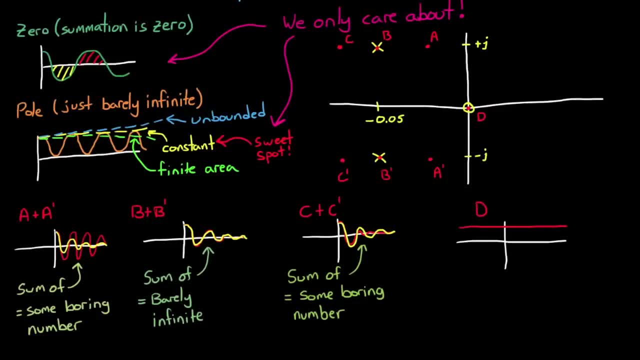 the probing function is just e to the 0, which is just a straight 1 across, And you multiply it by our impulse function, which will just be the impulse function, and you sum it all up: it'll cancel out and you'll get a 0.. 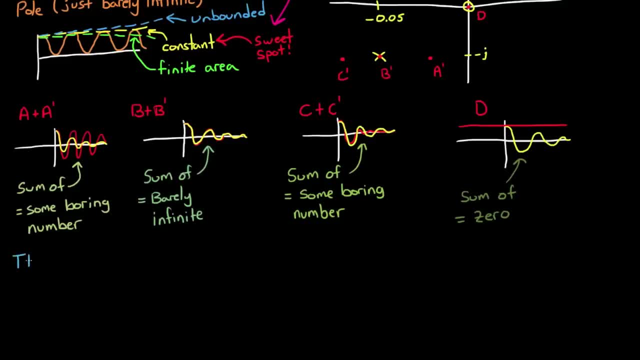 And once you take the Laplace transform of the impulse response and figure out where your poles and 0s are, you can generate the transfer function in the s domain by taking your 0s and dividing it by your poles. Remember, we have a 0 at 0,. 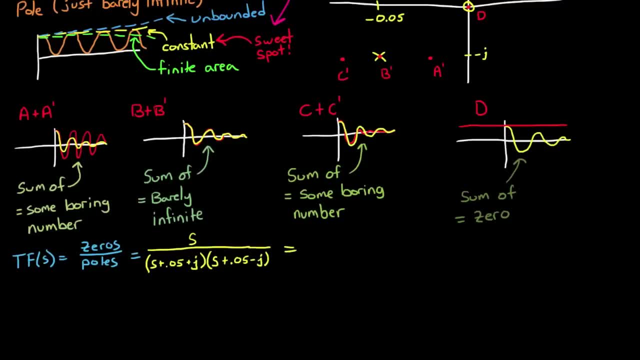 so that's just s and two complex poles which I've written here, And these can be multiplied out to be approximately s over s squared plus 0.1s plus 1.. And this is the transfer function of our system. But now we can take it a step further. 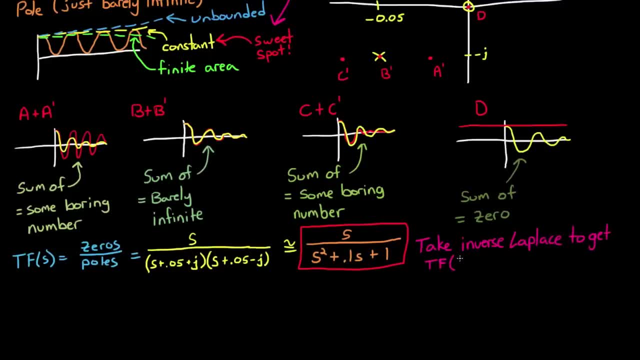 and take the inverse Laplace transform of this function to get it back into a time domain function. One thing to note about this process is that it's usually done in the reverse order. I did it in this direction because I think it makes more intuitive sense this way.